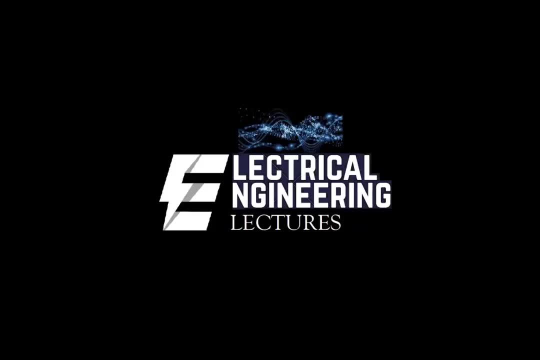 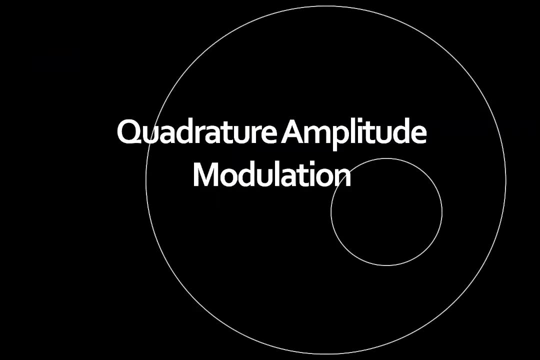 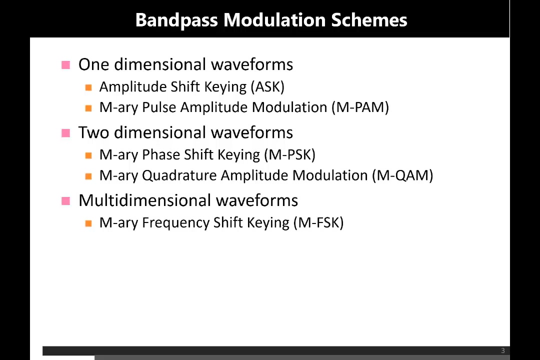 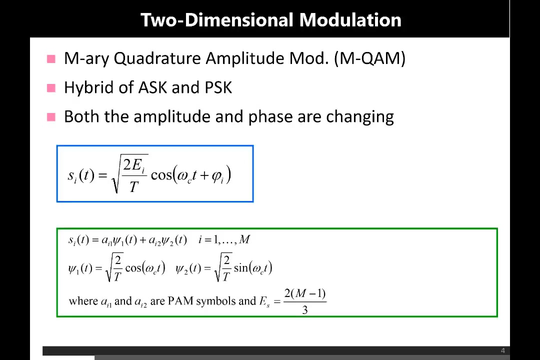 You are watching electrical engineering lectures channel. For more videos, please do like subscribe and hit the bell icon for the latest notifications. Thank you for watching Two significant words. The first one is quadrature and the second one is amplitude. This means that this modulation scheme is basically a hybrid of amplitude shift key and phase shift key. 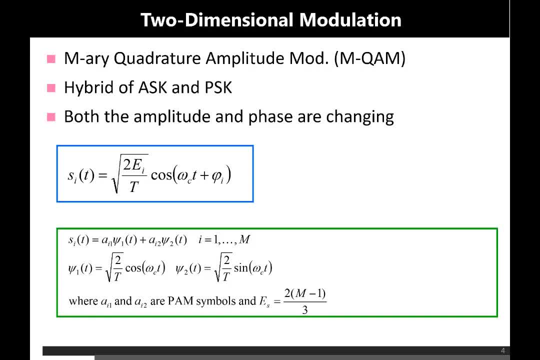 In other words, this modulation scheme changes the amplitude and phase of the carrier at the same time. So the information will be mounted not only the phase or amplitude of the carrier, but at the same time both the amplitude and the phase of the carrier. So the general expression for SI of T, the transmit pulse for the ith symbol, is given by this particular expression, as shown by this equation. 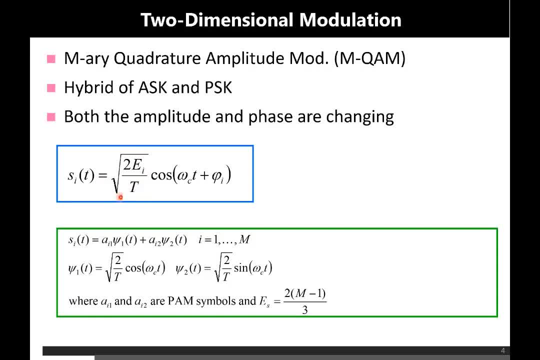 SI of T is equal to 2EI divided by T square root into cos, omega, CT plus phi I. So you see now the subscript I is appearing in both the amplitude and the phase of the transmit pulse, which shows that the amplitude is now is changing as well as the phase is also changing. So the information of the message signal or the bit stream is basically mounted on both the amplitude and phase. 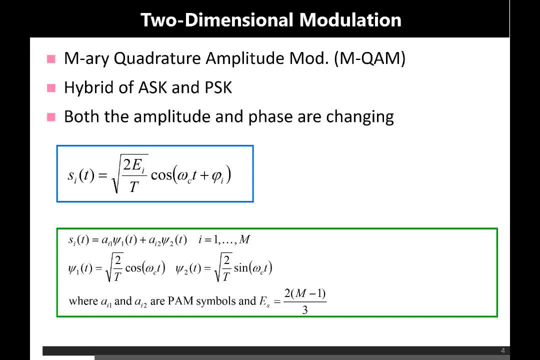 Now, in terms of basis functions, what is happening in case of quadrature amplitude modulation? We also abbreviate it as CLAM, So the transmit pulse expression in terms of basis functions will be the same as it was in the case of phase shift key PSK. 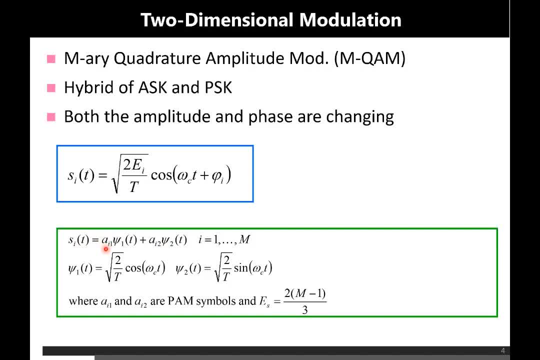 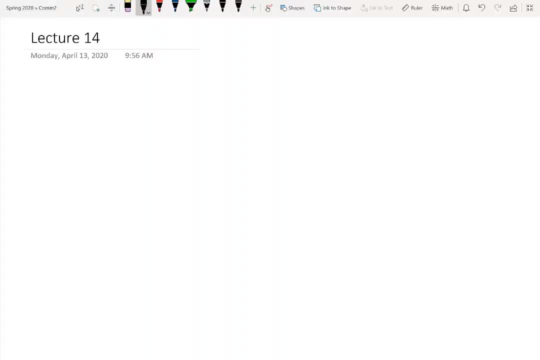 But now the difference lies in the fact that the coefficients Ai1 and Ai2, they are no more constants. They will be the function of the ith symbol, right? So to have a detailed explanation, let's come over here. I am writing here the equation for the ith transmit pulse again. 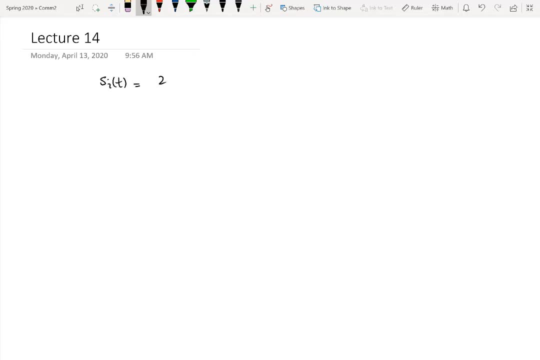 It will be: SI of T is equal to 2EI divided by T square root cos omega CT plus phi I, So let's call it equation 1.. And now the same transmit pulse in the form of basis functions can also be written as SI of T is equal to Ai1,. 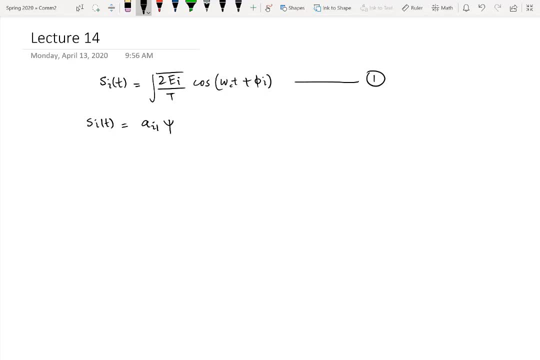 the first coefficient for the ith symbol into psi 1 of T, the first basis function, plus Ai2, psi 2 of T, the second basis function, Where psi 1 of T is, as a standard, given as 2 over T. 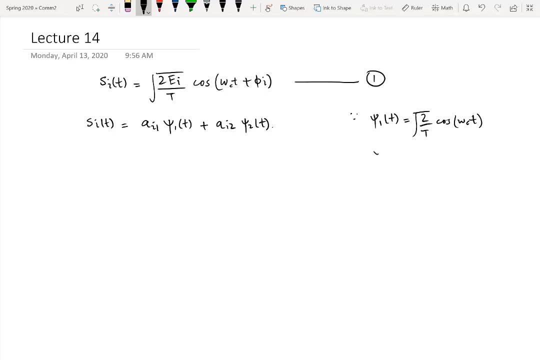 Cos omega CT and psi 2 of T is given as 2 over T, sin omega CT. So by using these basis functions and using equation 1, I can also write from here- I can split this SI of T by using the standard trigonometric identity as 2EI over T. 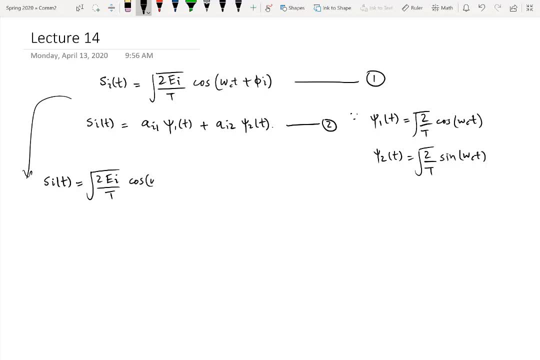 So I can write this: SI of T into cos omega CT into cos phi I plus sin omega CT into sin phi I Sorry, minus sign here, So now if I Sorry, minus sign here, So now if I Open up this bracket and rearrange the terms in one more step. 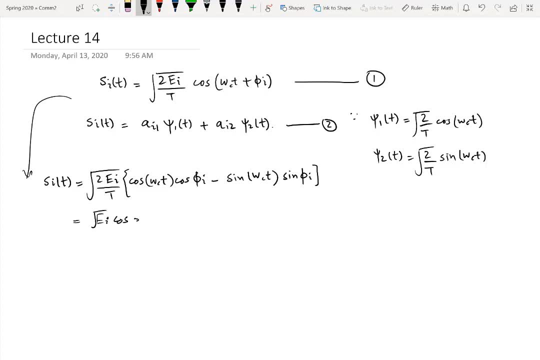 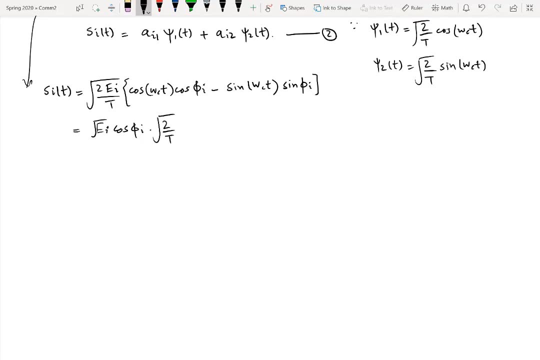 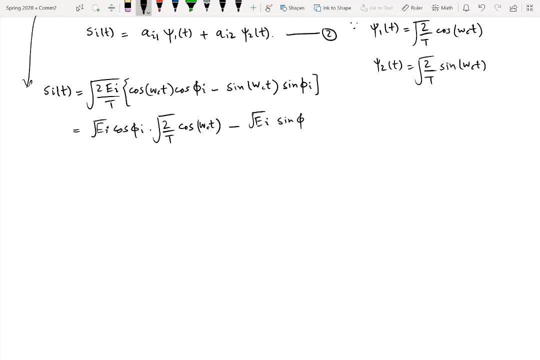 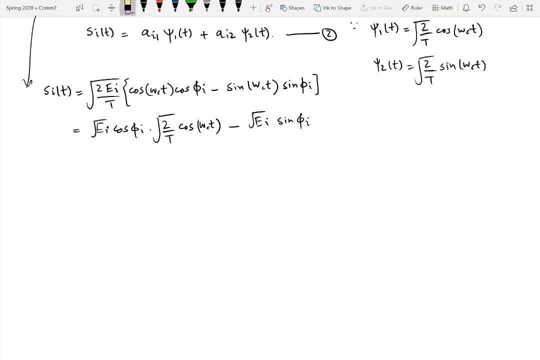 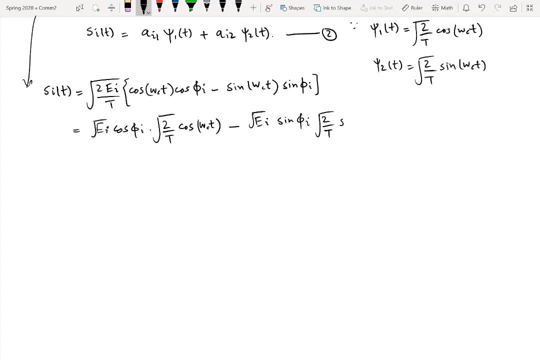 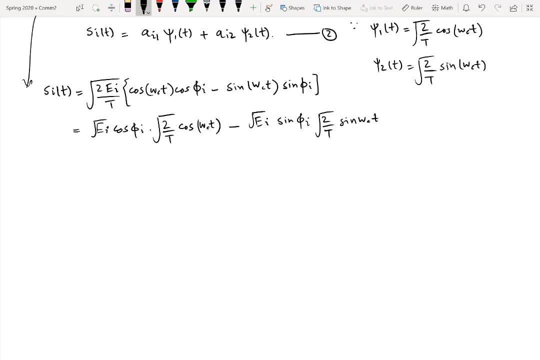 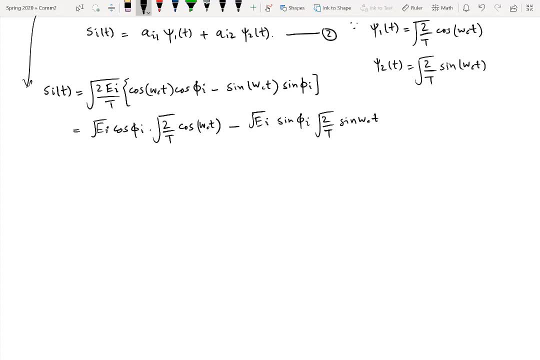 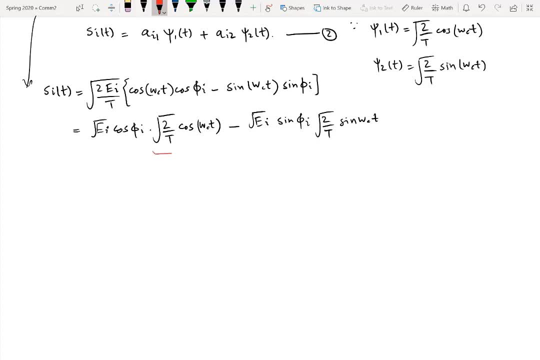 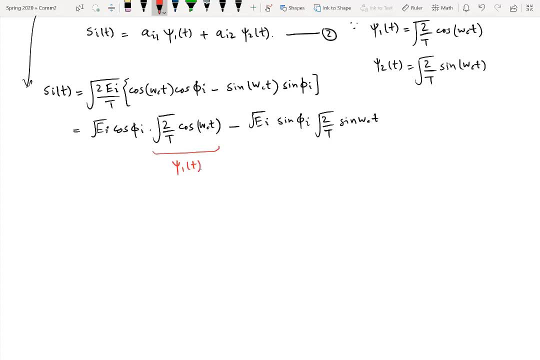 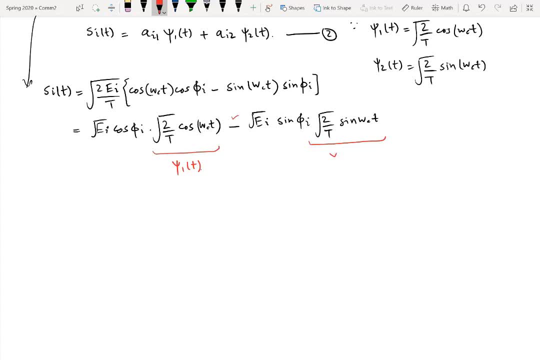 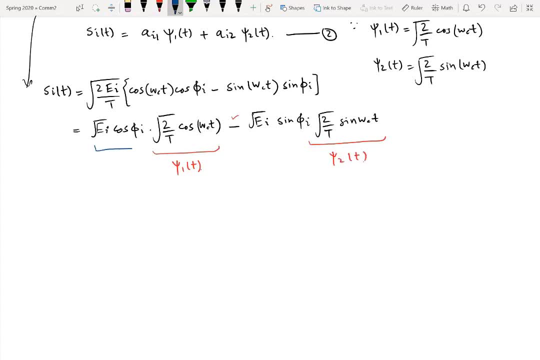 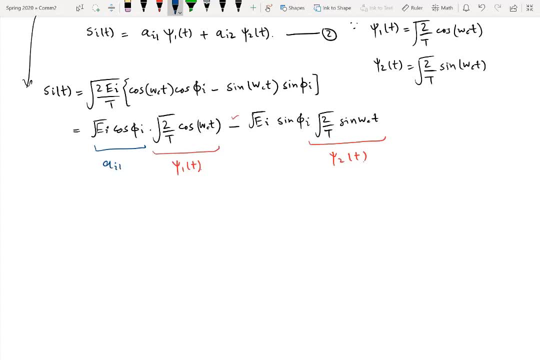 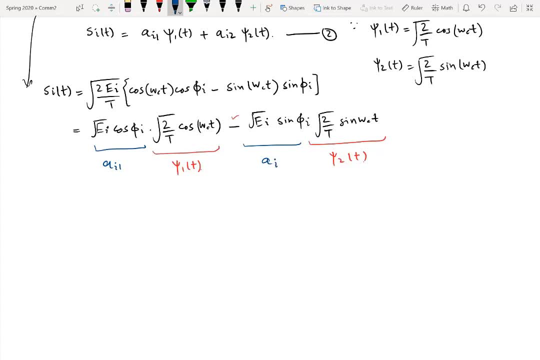 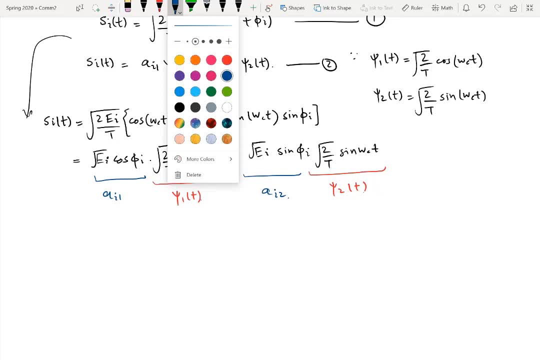 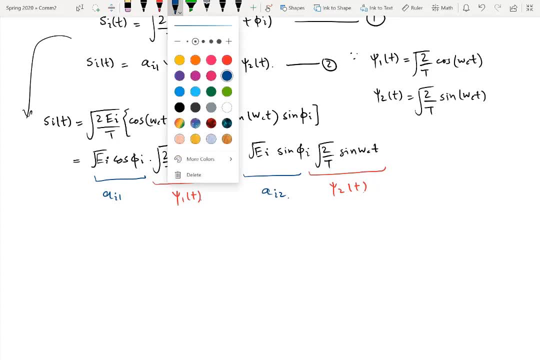 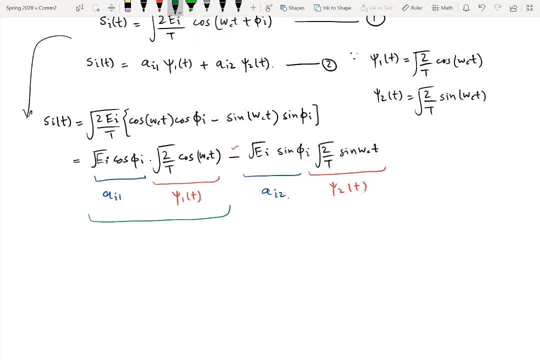 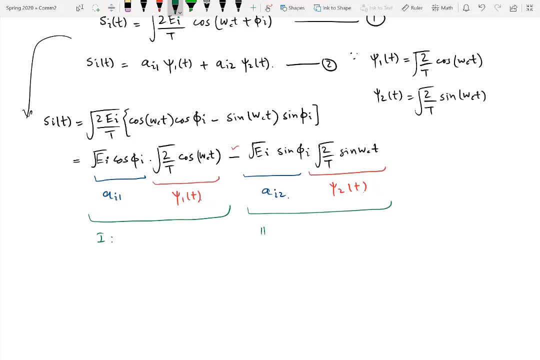 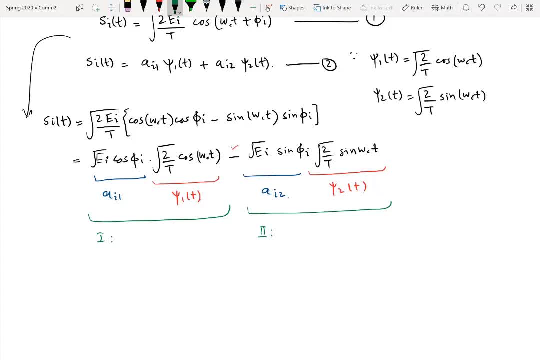 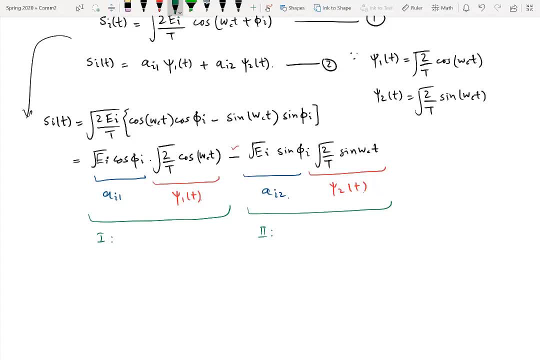 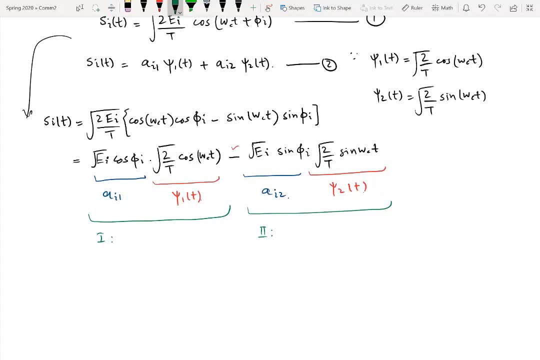 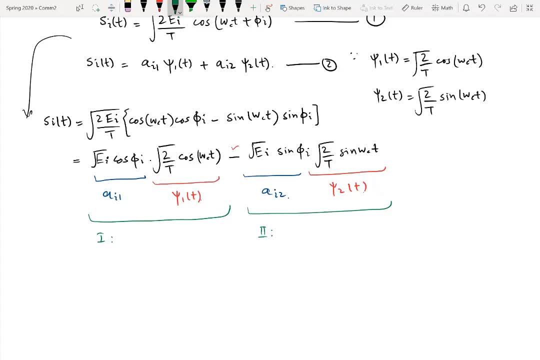 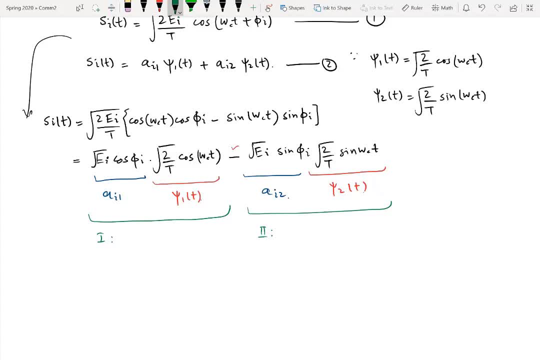 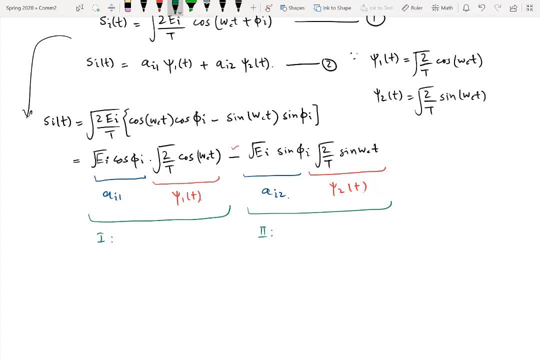 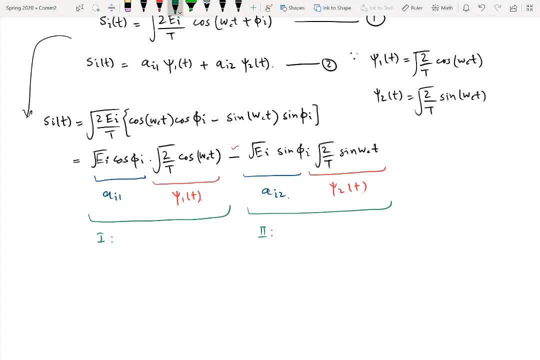 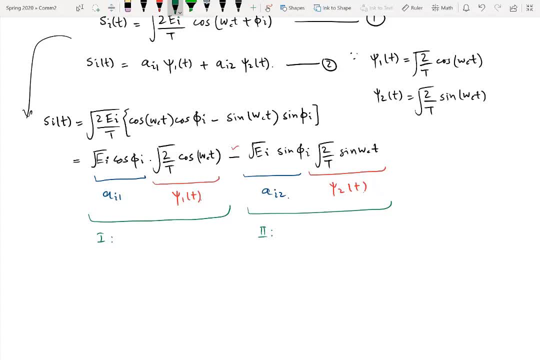 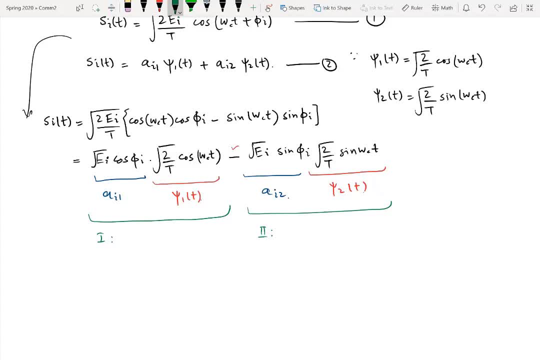 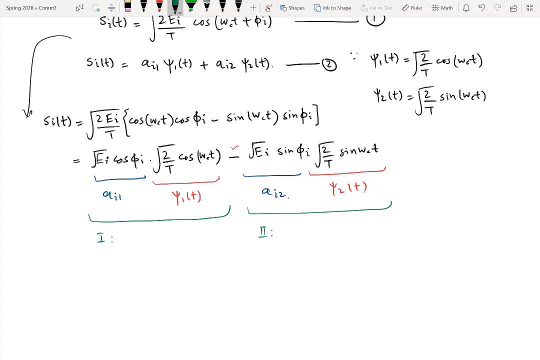 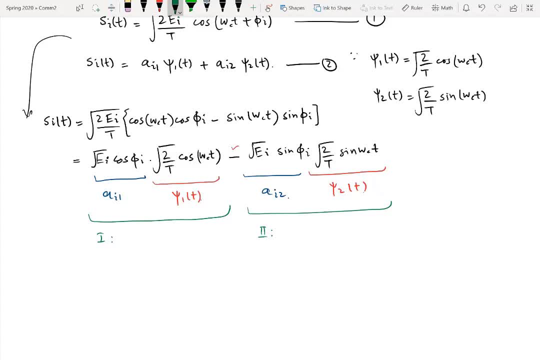 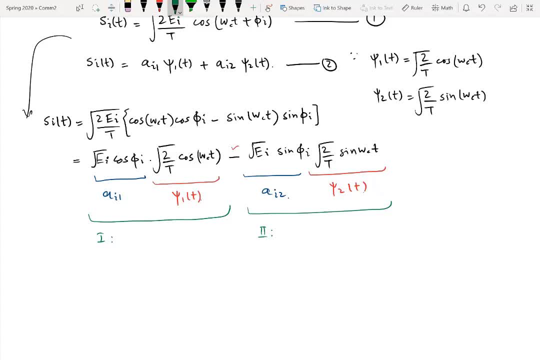 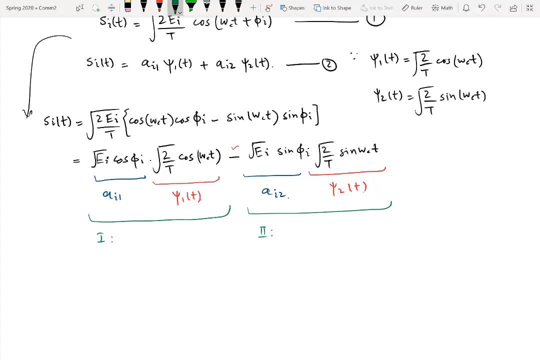 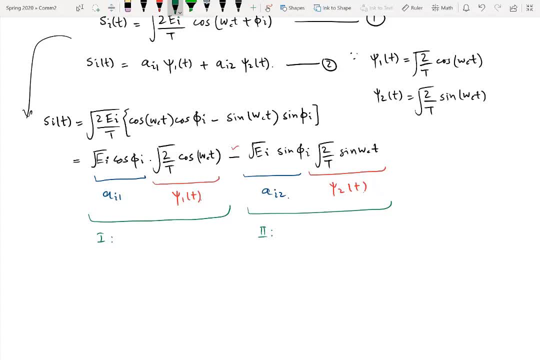 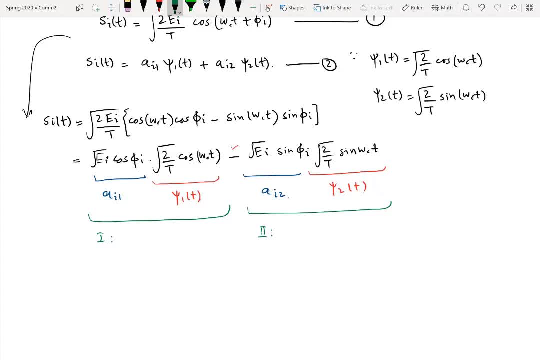 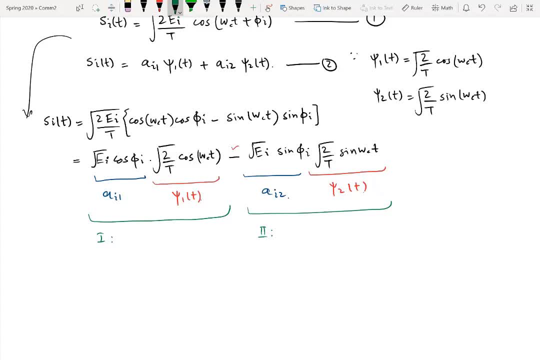 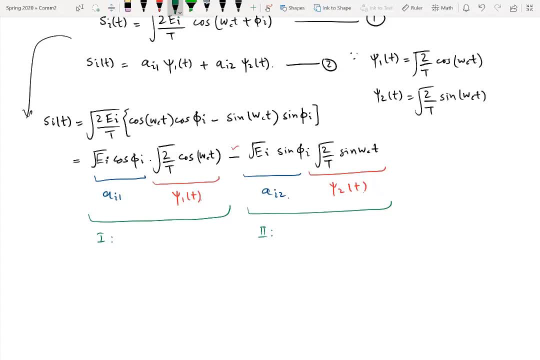 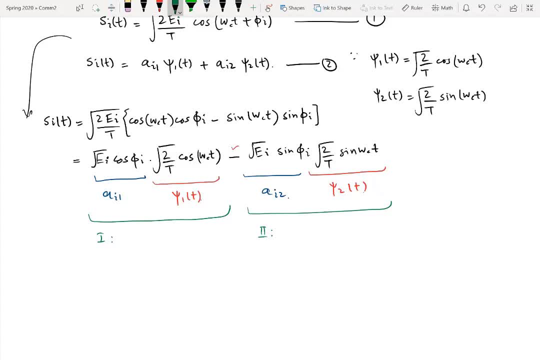 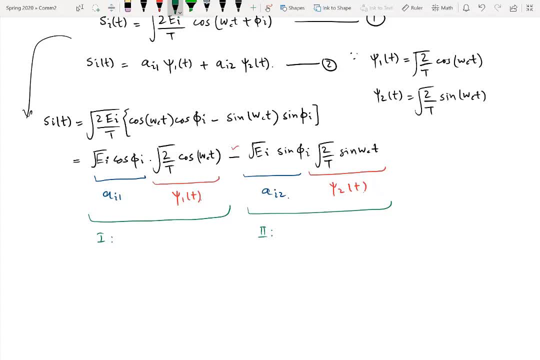 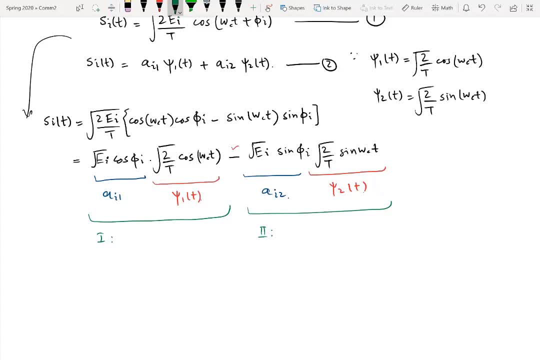 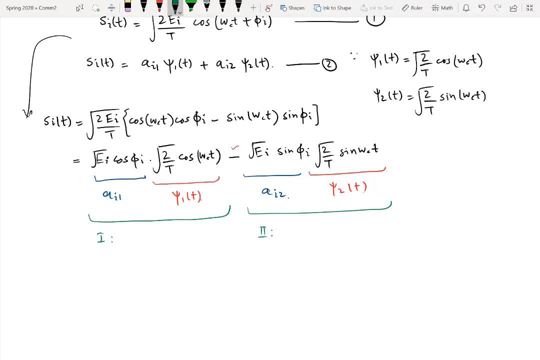 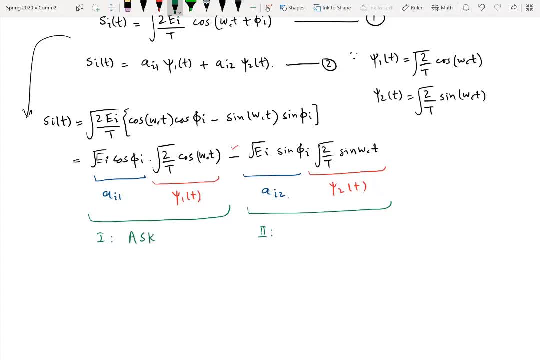 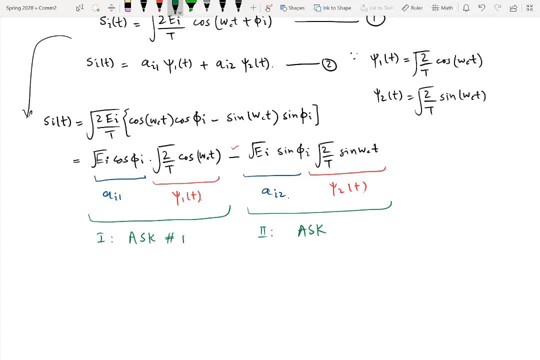 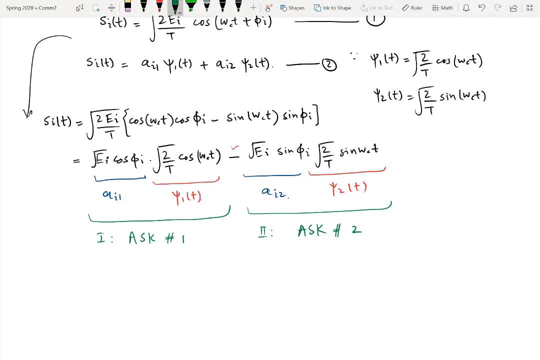 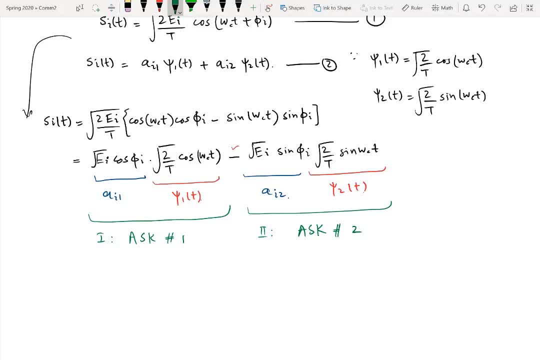 I can write as EI square root cos phi I multiplied by 2 over T cos omega CT, minus EI square root sin phi I scheme. we can transmit the data more more efficiently by using less bandwidth, because we are actually performing two types of modulations, and then we are 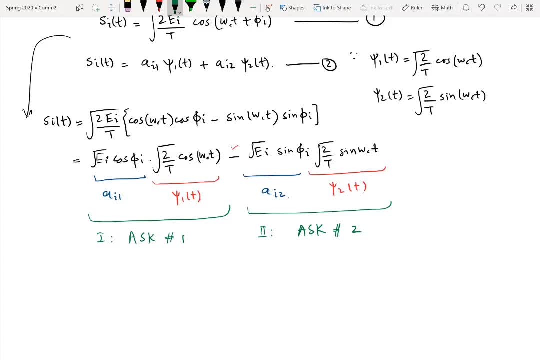 adding them up after the addition, we will transmit this signal. so in this way, this modulation scheme is more bandwidth efficient as compared to other modulation schemes, because by using the same frequency you are being able to transmit two different symbols. so this is symbol number one, this is symbol number two. so 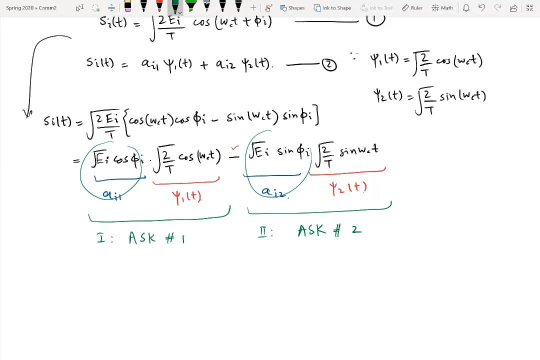 you are basically transmitting two different symbols over the same frequency. this is the difference. in previous modulation schemes- ASK, PSK- you were transmitting one more, one symbol on same on a single frequency. right here, you are able to transmit two different symbols at the same frequency simultaneously. that is why this modulation scheme is more bandwidth. 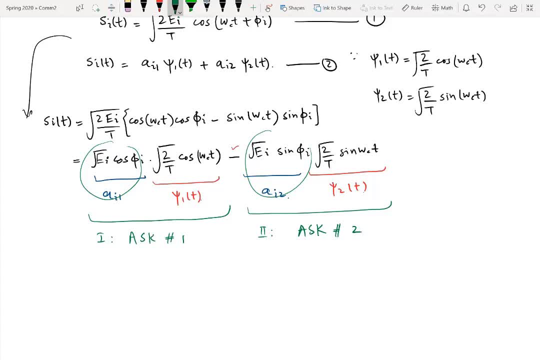 efficient and this is the reason why it's named ASKPSK. the name is quadrature, amplitude modulation. quadrature is due to the fact that the two carriers are quadrature to one another, and amplitude means we are basically performing amplitude modulation. so this is a brief. 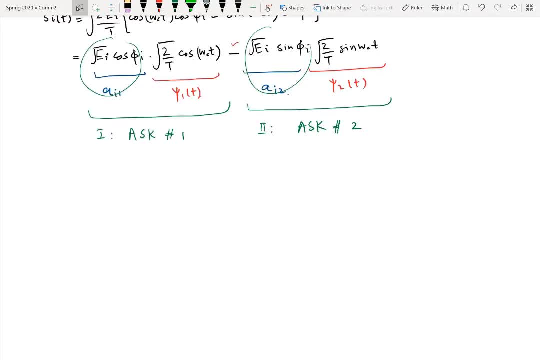 explanation of this particular concept, let us take an example. if we set M is equal to 4, we will have the values of AI1 and AI2. how we can have these values. so the general formulation to have these values will be M square root minus M. 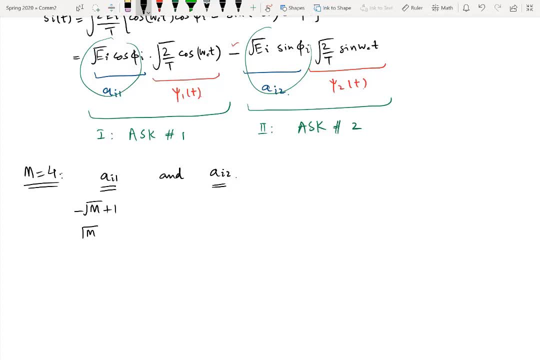 square root plus 1 and M square root minus 1. similarly, AI2 will also have the same values minus M plus 1 and M minus 1. so now you you see, we can have two values of the amplitude of AI1, and then M plus 1 and M minus 1. so now you see, we can have two values of the amplitude of AI1 and the. 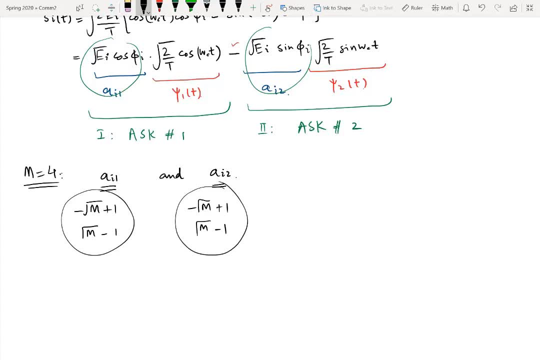 same two values of AI2. now we need to perform ordered pairs by using all the possible combinations, right? so it means that how can we formulate? first of all, this value will be combined with this one, and then this value with this one, then the lower value with this one and this value with this one. so it means we: 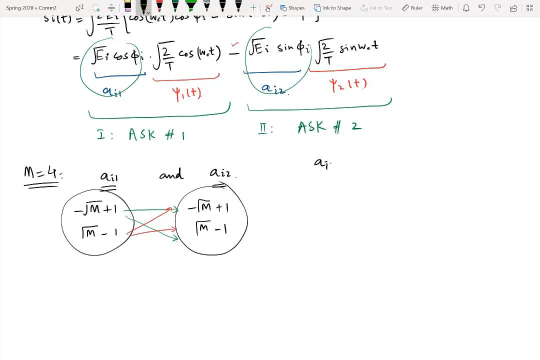 can construct a 2 cross 2 matrix over here in the form of ordered pair: AI1 comma. AI2 for m is equal to 4. I will have a matrix like this: minus m plus 1 comma, minus m plus 1. similarly minus m plus 1 comma, m minus 1 and here m minus. 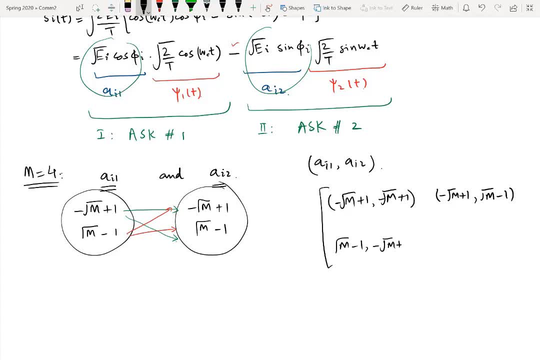 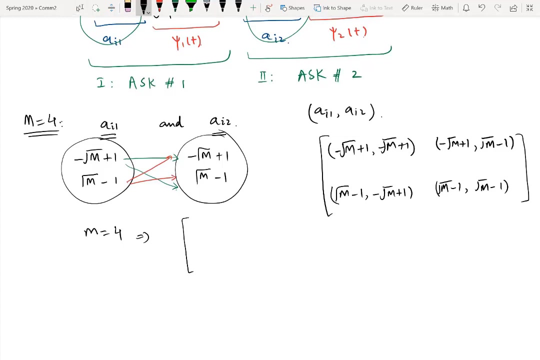 1 comma minus m plus 1. similarly here: M minus 1 comma, m minus 1. now for m is equal to 4. what's this matrix comes out to be? if you put just m is equal to 4 in the in this 2 cross 2 matrix, you'll be able to see that you are getting the following: 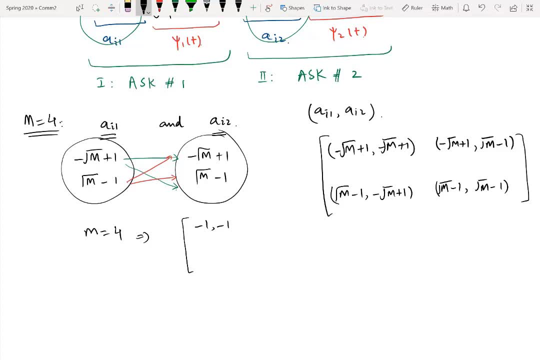 values you will be getting minus 1 minus 1, here minus 1, 1, here 1 minus 1 and here 1,1.. So these are basically the values of a i1 and a i2 in paired form right. So 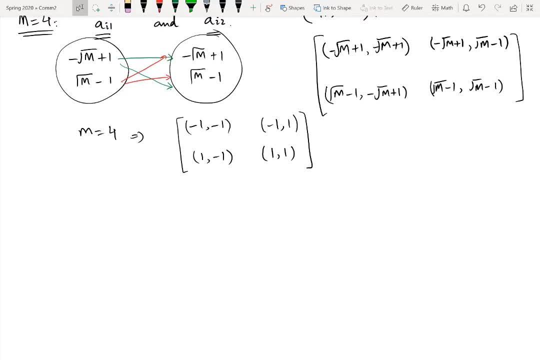 by using these paired values you can directly draw the constellation points, because I have told you in the previous lectures that the length of the constellation point or the magnitude of the constellation point is equal to the values of these coefficients. right? So it means now if 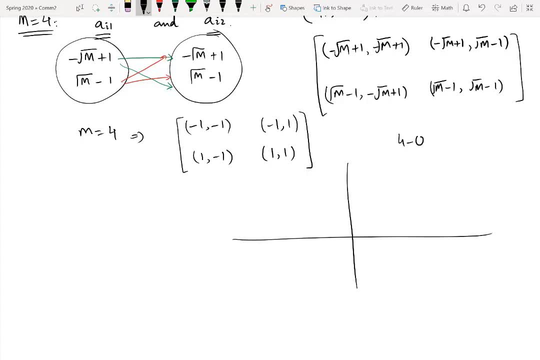 I draw the constellation of 4 co-m. 4 means m is equal to 4.. So this is real, this is imaginary. or you can say: this is psi 1 of t or this is psi 2 of t, because both are orthogonal to each other. 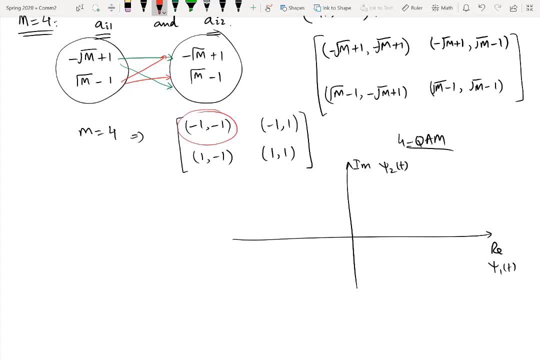 Now for the first ordered pair. let us say I select this one minus 1,1.. It means on the x-axis minus 1 and on the y-axis also minus 1.. So let us say this is minus 1,, this is 1,, this is 1,. 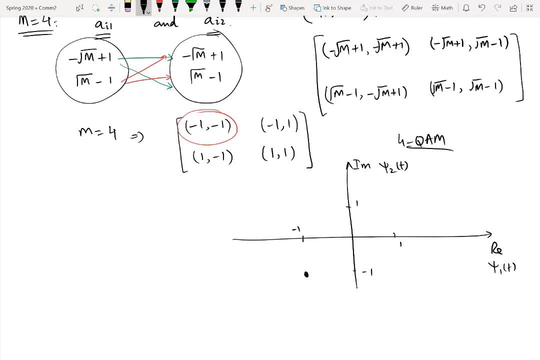 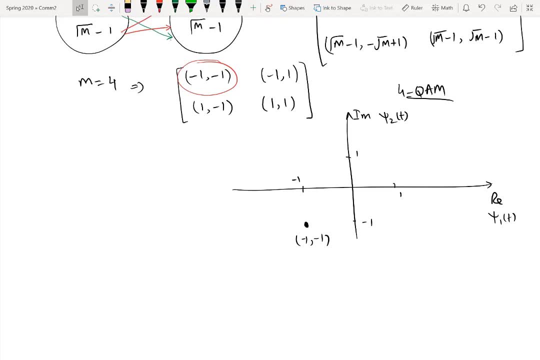 and this is minus 1.. So it means this point will lie over here: minus 1, minus 1.. Similarly the second one, minus 1,1.. So on x-axis minus 1 and y-axis 1.. So it will be this point. 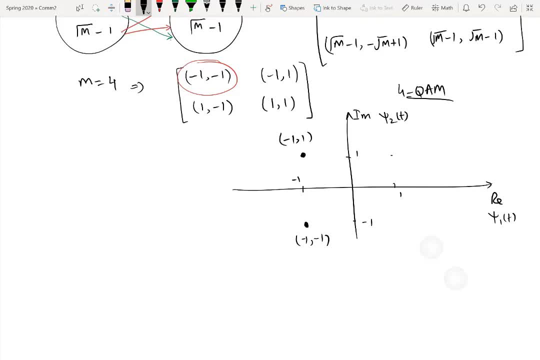 minus 1,1.. And similarly, if you plot the other two points, you will get these two points: Here it is 1,1 and here it is 1, minus 1.. So these are basically the four constellations of a i1 and a i2 in paired form, right. So by using these paired values, 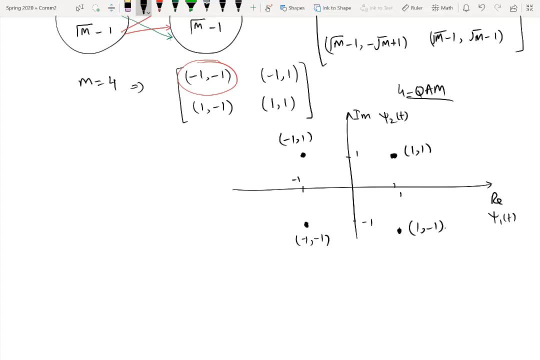 you can write the constellation points of quadrature. amplitude modulation for m is equal to 4, right. So in this way and in the form of bits, you can always write them in any fashion. but by using gray coding you can write 0,0,, 0,1,, 1,1, and 1,0 or any other notation. 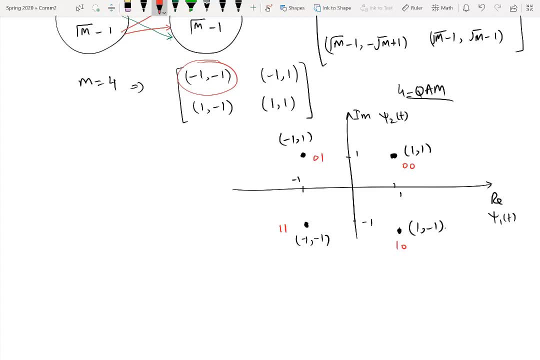 So this 4-quam is very much similar to QPSK: quadrature phase shifting. There is no difference in terms of bandwidth efficiency. But if you increase the value of m- and usually for QAM we make m as the multiple of 4, right, the multiple of 4.. 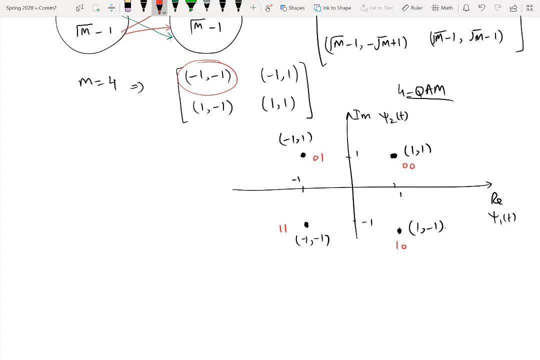 So it means the next value of m will- be sorry, in the power of 4.. So instead of in the power of 2, we select in the power of 4.. So the next power of 4 value will be: m is equal to 16.. 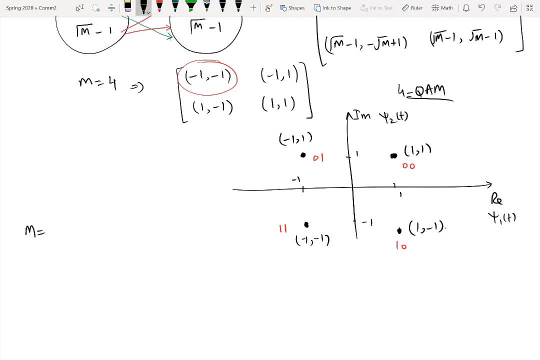 So if you select, m is equal to 16. now, for m is equal to 16,. what are the possible values of a i1 and a i2?? First of all, we have to know the possible values of a i1 and a i2.. So we have to. 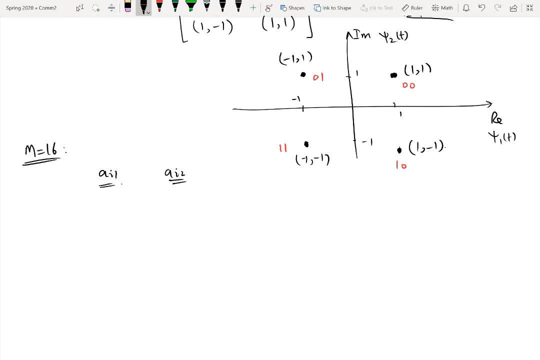 know the possible values of a i2.. So we have to know the possible values of an i1 and a i2.. So first of all we need to identify these values and the general formulations is that you select the values such that they are underscore m minus 1, minus under root m plus 1, then m minus 3 and. 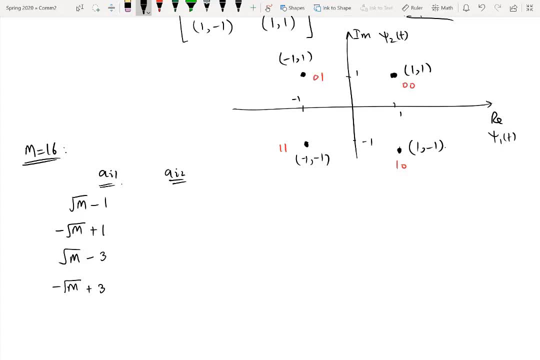 minus m plus 3.. So now it will have four values. So it means that the number of values for each coefficient will be log 2 of m. In this case it will have three values. So we have to do the following. 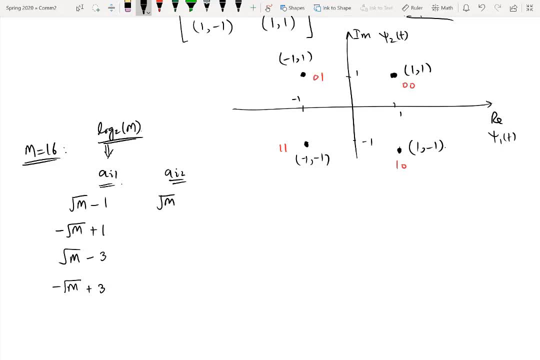 it will be 4 and the same values will come over here: under root m minus 1, minus. under root m plus 1, under root m minus 3 and under root m plus 3 with minus. so again, by using these four values and these four values, you will perform ordered pairs and in at this time you will get a 4 cross. 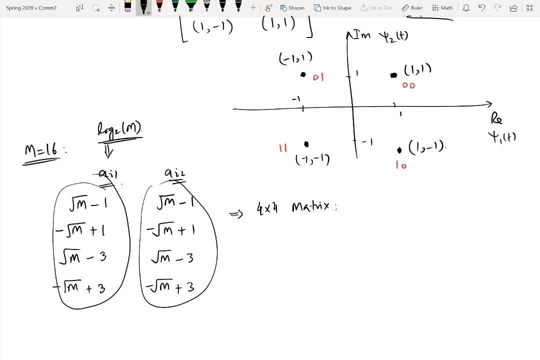 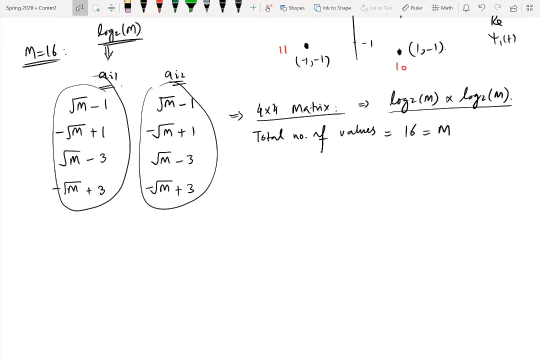 4 matrix. so the total number of values, total number of values, will be 16, which will be equal to M, and the size of the matrix will be log 2 M, cross, log 2 M, point. so now, if you directly calculate the values, as in that case, we have got a 2 cross 2 matrix and in this particular case you will have 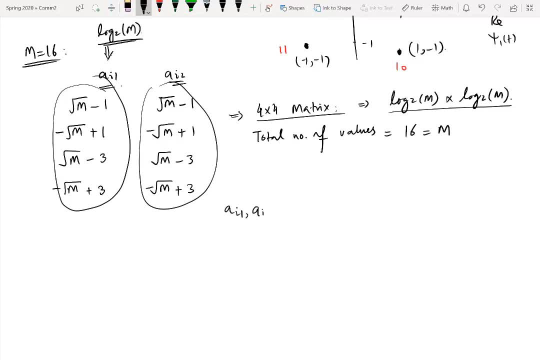 4, cross 4 matrix like this: a i1, a i2, and it will be in the form of this matrix containing minus 3 comma, minus 3, minus 3 comma, minus 1, minus 3 1 and minus 3: 3. similarly, you will: 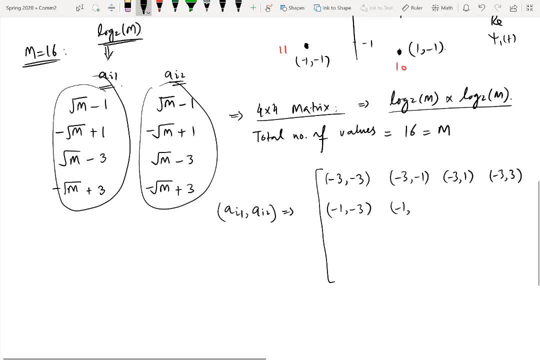 have minus 1 minus 3, minus 1 minus 1, minus 1- 1 and minus 1- 3. then you have 1 minus 3, then you will have 1 minus 1, 1, 1 and 1: 3 and the last row will be minus 3. last row will be 3 minus 3. 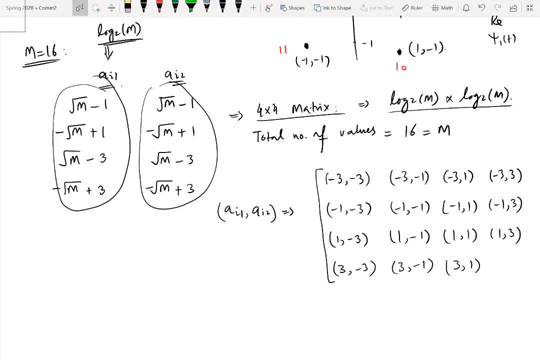 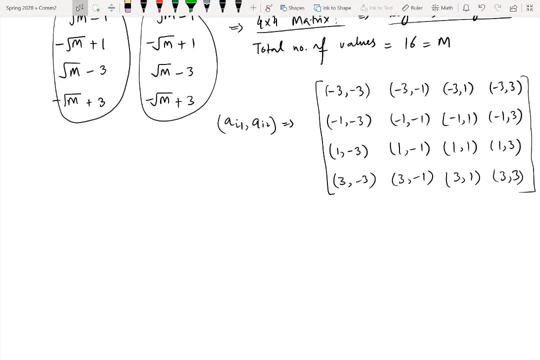 3 minus 1.. 3, 1 and 3- 3, so this will be the 4 cross 4 matrix containing 16 ordered pairs containing the values of AI 1 and AI 2, so by using these values, because these are the magnitudes of all the constellation points. so now, if you draw, 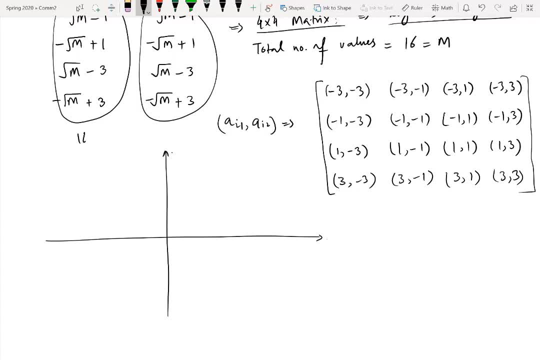 the constellation point. constellation diagram for 16 QAM. because M was 16, so for 16 QAM it will become. it will contain how many, how many points? it will contain 16 points now in this formulation, so four points in each quadrant. so this is basically the constellation diagram. 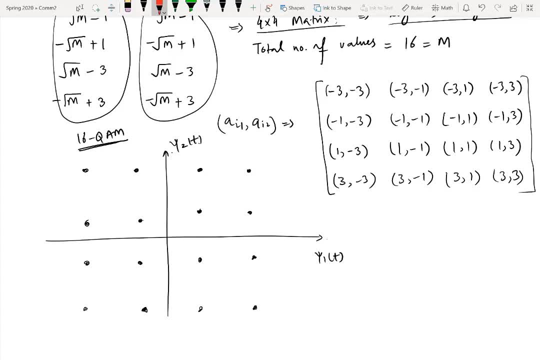 for 16 QAM, for example. as an example, I am just writing coordinates of a couple of points. for example, this point has the coordinates 3 comma 3. if I write the coordinates for this particular point, they are minus 3 comma 1. let's say, if I write the. 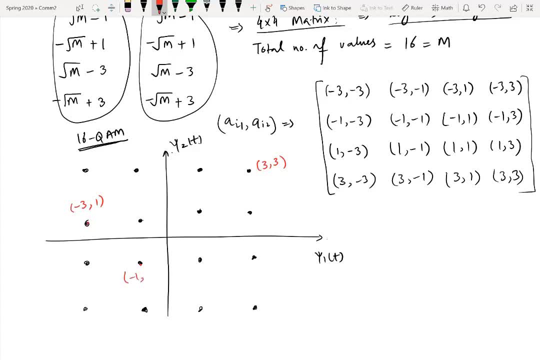 concentration point. for this one, the coordinates, it will be minus 1 comma minus 1. so in this way you can easily find out the coefficients in the coordinates of all the points. so that this point is 1, this point is 3, this is minus 1. 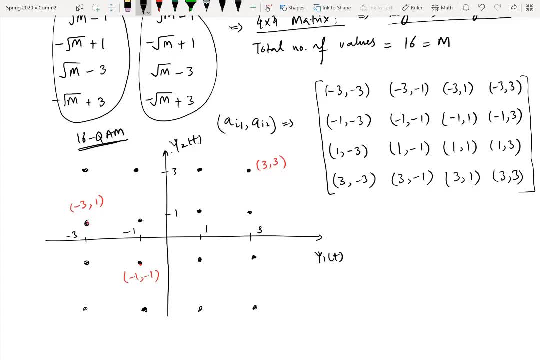 this is minus 3, 3, 1, minus 1 and minus 3. so you see, if you now observe this particular constellation diagram and compare it with either amplitude shift key or phase shift key, by keeping m is equal to 16. so if you keep, m is equal to 16 and 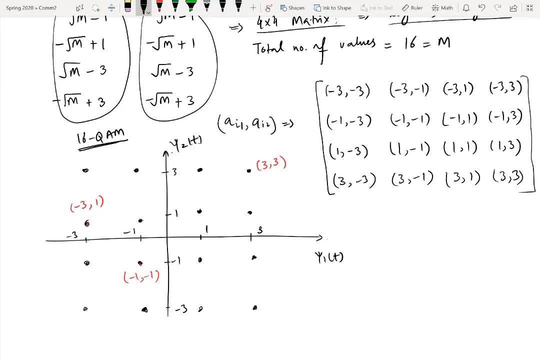 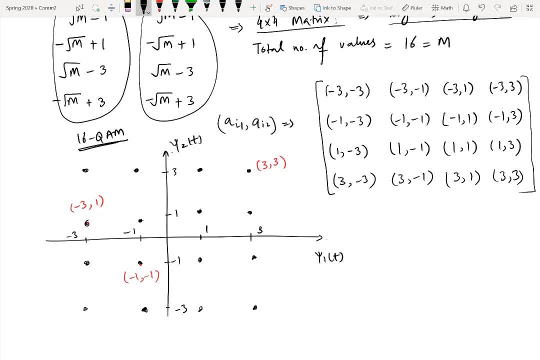 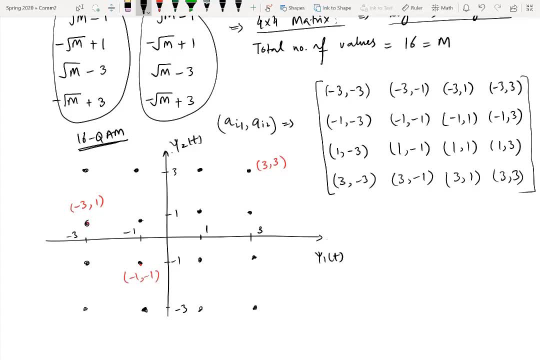 all the 16 points will remain the same, magnitude will remain the same. the only thing changes is the phase. but here, in case of 16 QAM, you are observing that both the amplitude and phase are changing. for example, if I take four points in one quadrant and let's consider this point, so this point, 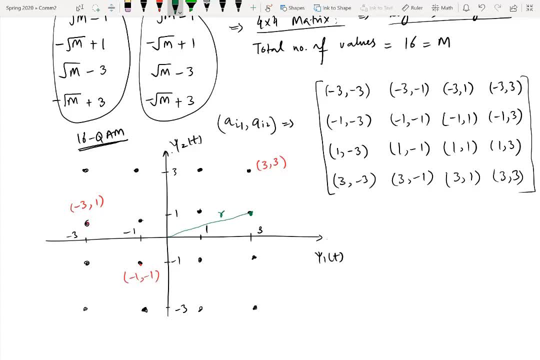 has a radius, let's say R, and that radius is exactly equal to this radius. but what is the difference? the difference is the phase right. similarly, if you take another example, and I say that this point is, it has a radius r1 and this point 33, it has got the radius r2. so here, what is the difference? 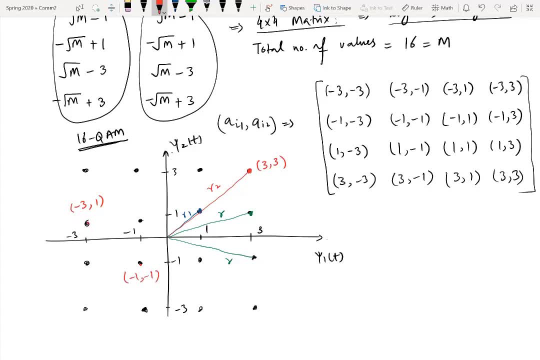 the angle is the same. but what is this? what is the different thing? the different thing is the magnitude. the magnitude of first one is r1 and the second one is r2. so, in this way, this constellation diagram is a mixture of amplitude shift keying and phase shift keying and, due to 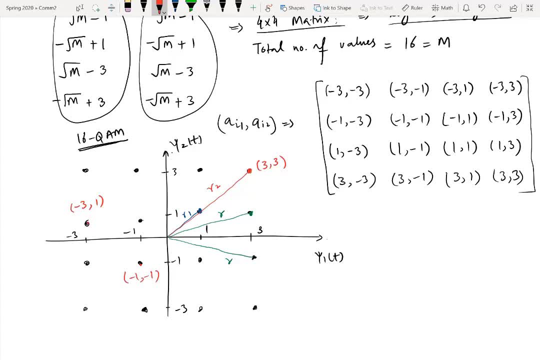 this reason. this is bandwidth deficient and at the same time, the performance of 16 qam will be better as compared to 16 psk. we will see in the upcoming lectures. when we compare the der performance of all these modulation schemes, we will see that the performance of 16 gram is much. 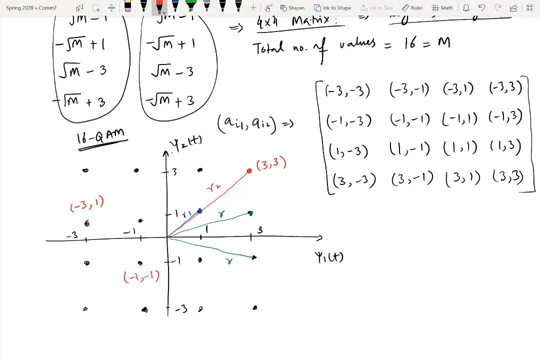 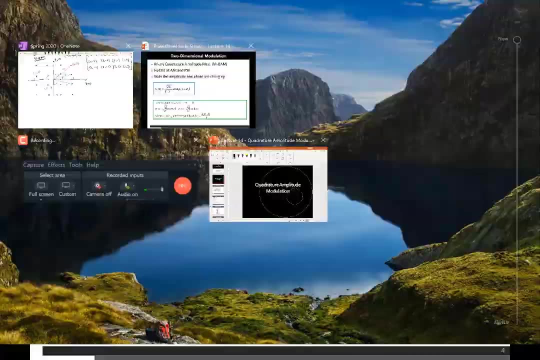 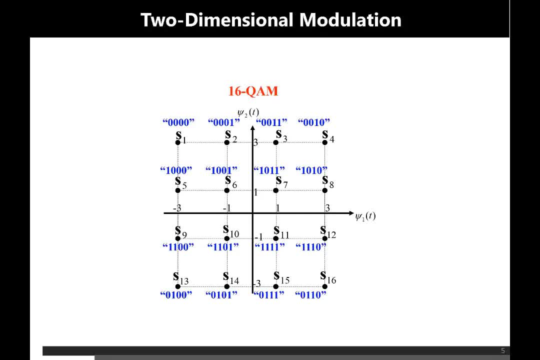 and for, definitely for 16 gram, the number of bits per symbol k, it will be equal to 4, so each constellation point or each symbol will be corresponding to 4 bits and definitely there will be 16 combinations. so you can follow any scheme to allot or to allocate the these symbols. 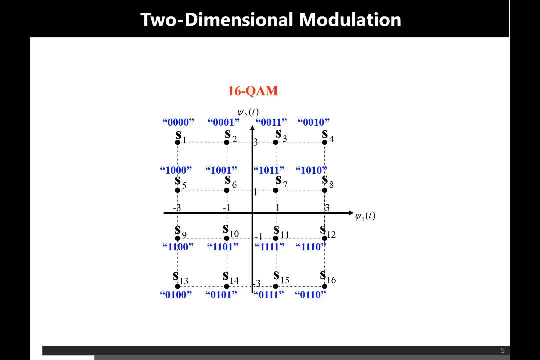 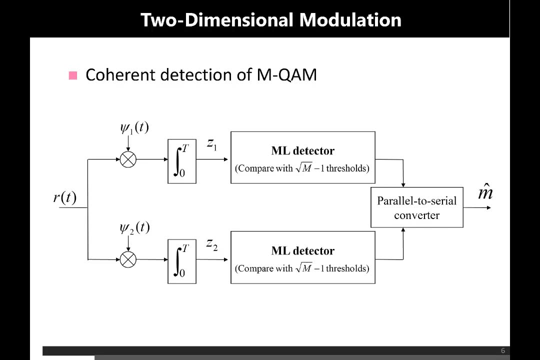 to any constellation point but it is assumed that you will follow the this scheme and the gray coding so that they each consecutive symbol for each consecutive symbol we have the observe only 1 bit now we come towards the coherent detection of this mary or mqam now before discussing this block diagram you need to understand a very basic point and you need to recall that point that i have told you in the start of the lecture that this qam is basically � Hooke and you need to recall that point that i have told you in the start of the lecture that this query is basically 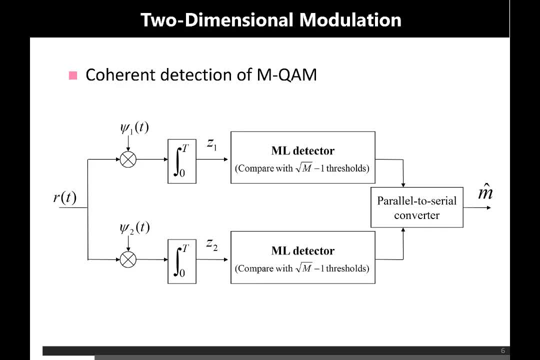 combination of two amplitude shift keying schemes, one amplitude shift keying being performed with cos omega CT and the other amplitude shift keying being performed with sine omega CT right. so it means that it is a combination of two ASK. and when it is a combination of two ASK, it is a very intuitive to understand. 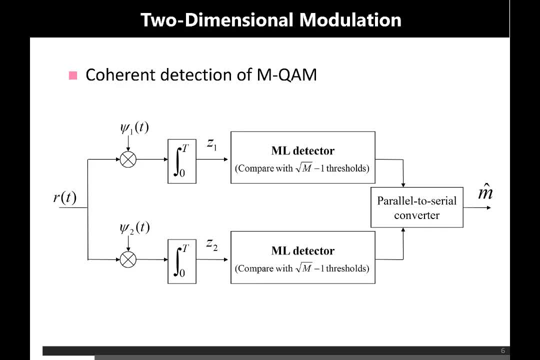 that we can formulate the coherent detection of QAM by just combining two coherent detectors of amplitude shift keying. and we just combine them and we place them in parallel because, if you recall, for amplitude shift keying we only require one basis function. so we will just use two coherent detectors for ASK and 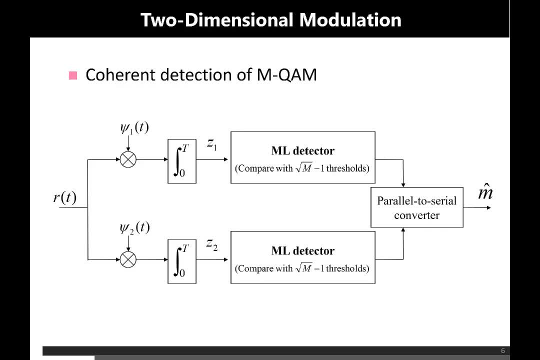 place them parallel. one ASK detector will be using psi 1 of T, which is made of cos, and the second one is made of which. in second, one will be using psi 2 of T, which is actually made up of sine omega CT. so it means: 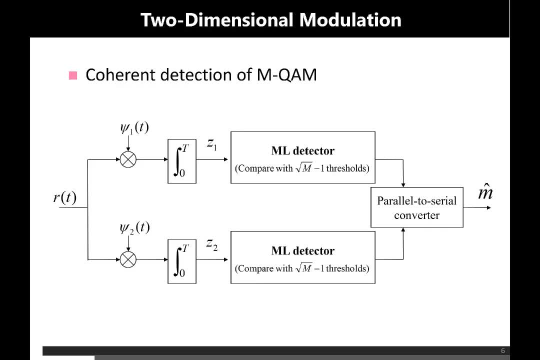 a, a, a, a. this is a very simple architecture. so you see, now the incoming singular is R of T. by using this R of T, we have two types of. we will have two branches. this is the first branch and this is the second branch. so you can say that this 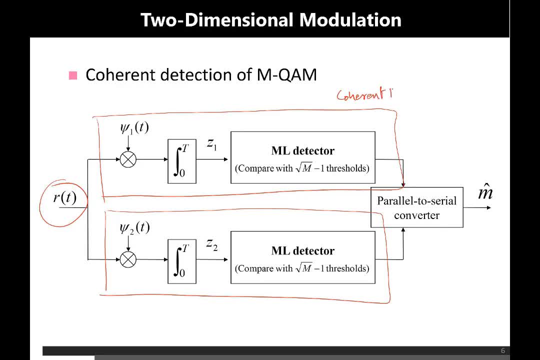 is coherent detector for ASK1. that was shown in the derivation and this is coherent detector for ASK2. the only difference is this is governed by Psi2 of T and the first one is governed by Psi1 of T, so it was made up of. 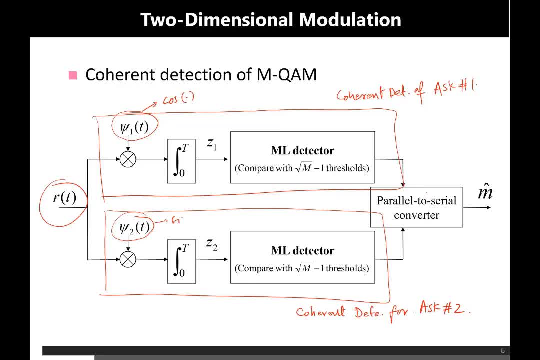 cos and this is made up of sine and they are quadrature to each other. so you simply see the same effect occurring over here. so the received signal will be multiplied with Psi1 of T and in the second branch it will be multiplied with Psi2 of T. 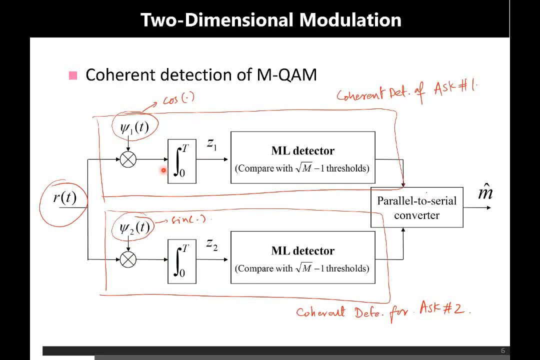 like here. and the next stage is the correlation, as it is a mandatory part of all the all the detectors. it is coherent, it is basically performing correlation and the output is Z1 and Z2. this Z1 and Z2 will be fed into the thresholding, or 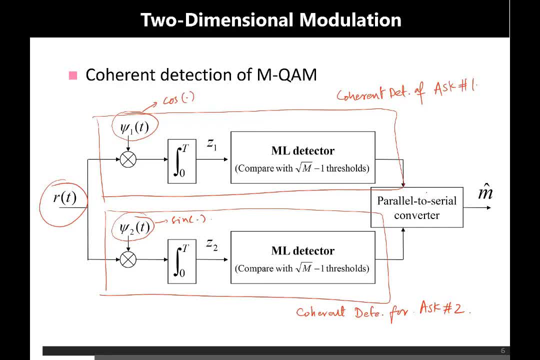 detection stage. but now you have got two coherent detectors working in parallel. now the question is how many thresholds each of these detectors will be using, because in the previous cases we have discussed that the number of thresholds are equal to M minus one, but here there is a slight 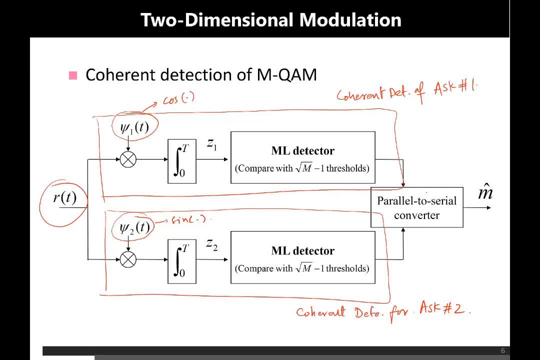 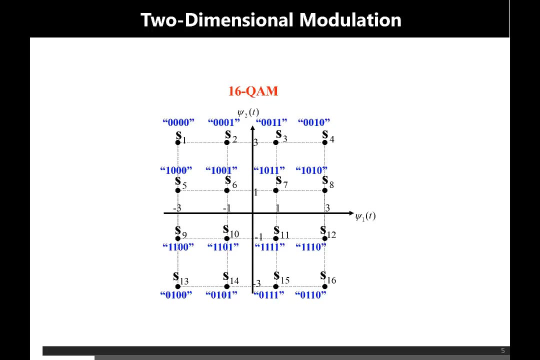 difference. you see, here it is written that, compared with square root, M minus one detectors. now, what is the difference? why we are not using M minus one detectors over here to understand this concept, let's come towards this constellation diagram. if you see, if you are going to find, because each of these 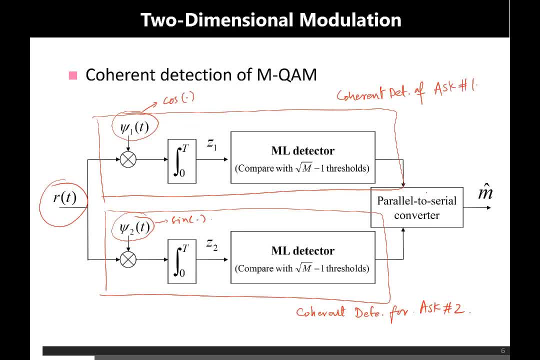 branches. each of these branches is a separate amplitude shifting detector, so separately. so it means, if we find out that how many magnitudes are, how many amplitudes are existing in this constellation, we simply be able to find the number of thresholds right. so how many different amplitudes are available? 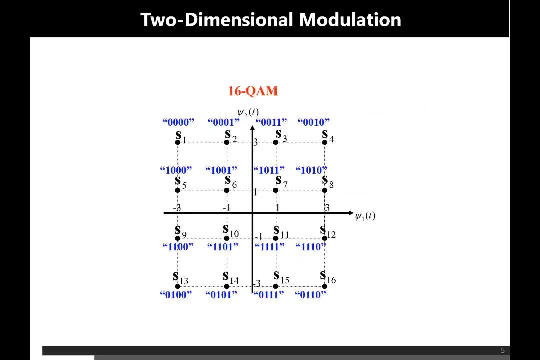 in this constellation diagram. you see, now you come over here, the first magnitude is this one and this magnitude and this magnitude. this magnitude and this magnitude are the same, so you call it number one. the second one is this point: s4 for s16, for s13 and for s1. so all these magnitudes are the same it. 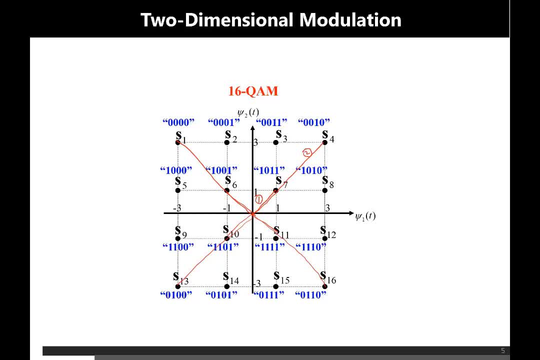 means let's call it magnitude number two. and the third one is this one, here, here, here and here, and also this one, so these eight constellation points will have the same, will have the same magnitude. let's call it number three. so it means we have got three different. 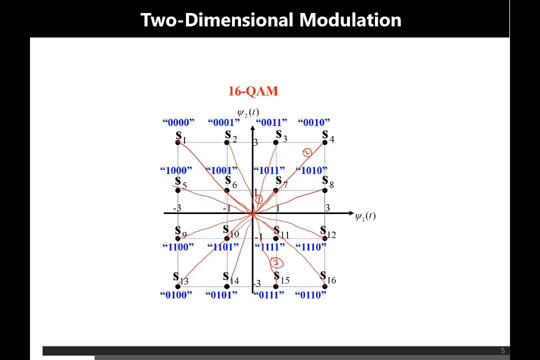 amplitudes all over this constellation diagram in terms of energy, or you can say that the number of possible energies is basically three. so when it is three, it means, if we relate it with the value of m, you can say that the number of possible energies is basically three. so when it is three, 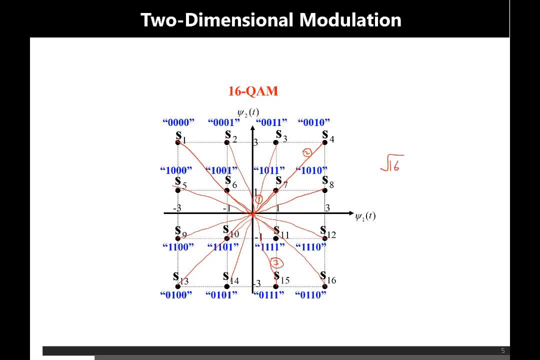 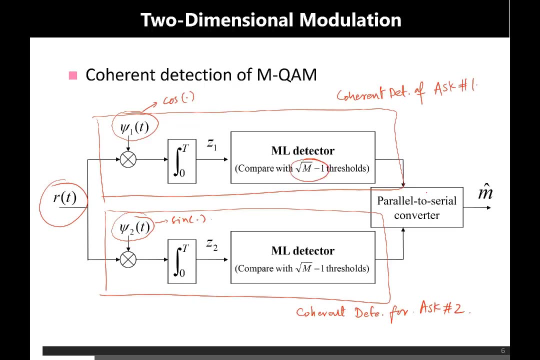 we can say: because this is for 16. so if I write 16 square root minus one, it means m square root minus one, which comes out to be three. we need to have three different thresholds for each branch right so that the same thing is written over here, because each detector is a separate amplitude. 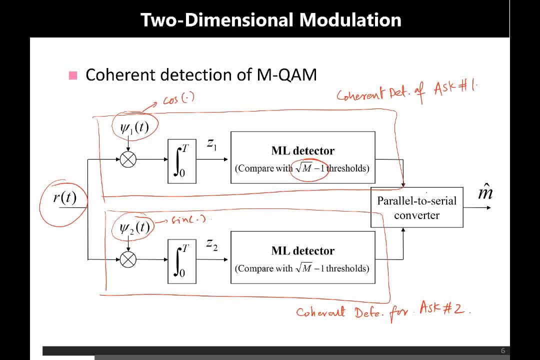 shifting detector. therefore, each detector will be using under root m minus one thresholds. you can also verify it: for m is equal to four. because for m is equal to four, you will answer will be under root m minus one, equal to four minus one, and that will be equal to one. so 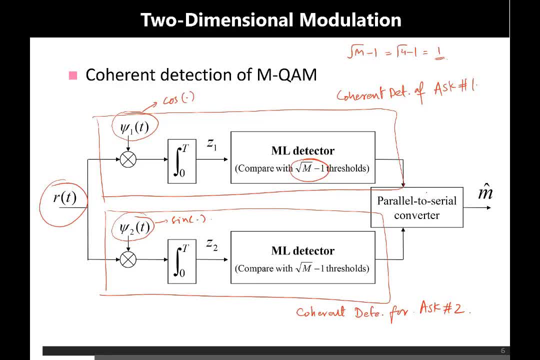 you can only read one threshold. one threshold means there is only one magnitude all over the constellation for m is equal to four. so that is the reason why we are only using under root m minus one thresholds inside each detector and this is the reason why quadrature amplitude modulation. 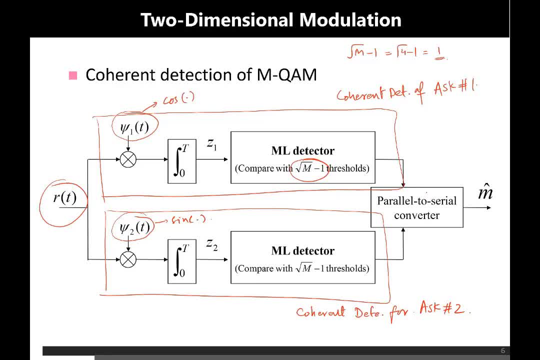 modulation is performing better. it will perform better as compared to other schemes because in 16 PAM you take, m is equal to 16 in PAM you will require how many thresholds? 15 thresholds, m minus one. you will require 15 thresholds, so there will be more chance of errors. but here in total, how many? 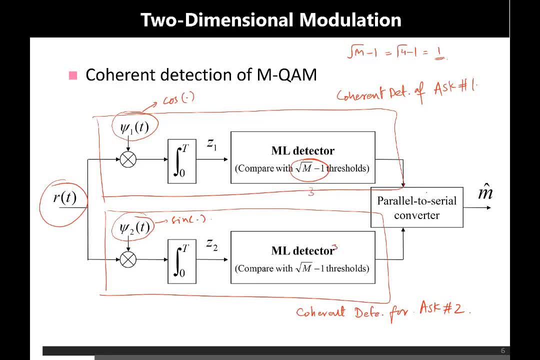 thresholds are being used, three here and three here, for m is equal to 16, so total of six thresholds. it means you can have less probability of error because of less decision regions, because more the number of decision regions, more the probability of error. here you will experience less probability of error and after the output of this, these two separate.